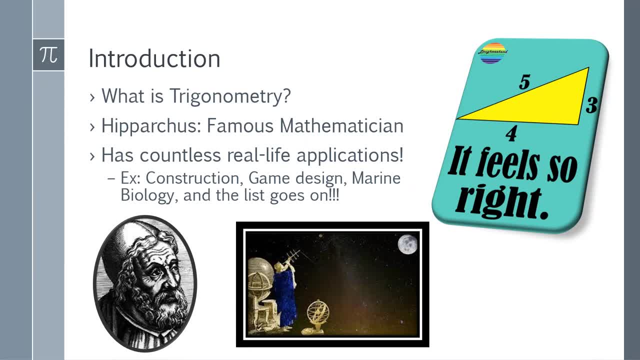 a table of values for trigonometric functions, which is still in use today. Since he had a strong passion for astronomy, he had actually used trigonometry to make his calculations much easier by using methods to solve for spherical triangles using the table of values that he had constructed. Although Hipparchus had done all this work for society, 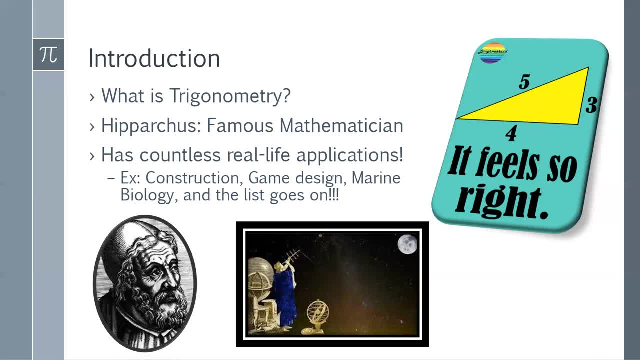 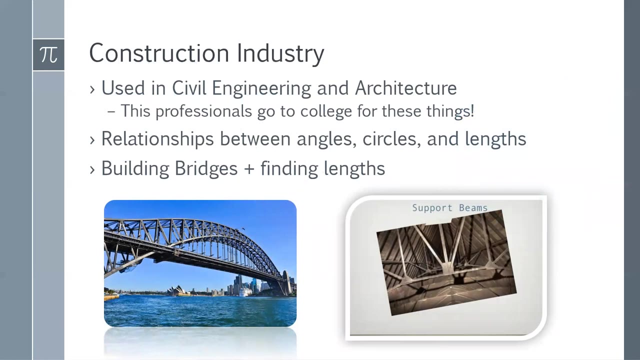 modern and advanced technologies has actually allowed us to use trigonometry in the real world. Therefore, the construction industry, the creation of video games and the development of marine biology are perfect examples that show trigonometry in real life. So the construction industry, that should be something that's really important to us. 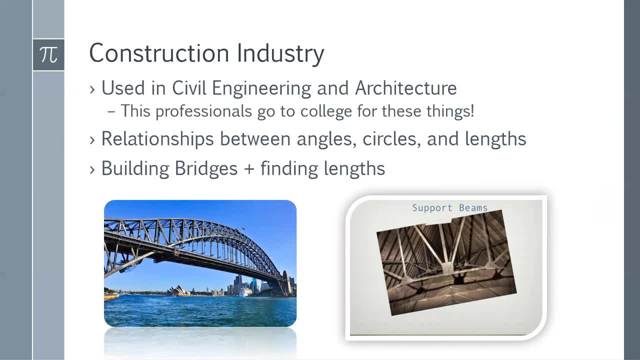 because those individuals that are working in this industry are the ones that are creating different buildings, bridges and many more. A lot of these people are actually architects and civil engineers, and these people go to college for a really, really long time just so they get experienced and certified Architects. they use the trigonometry to calculate structural 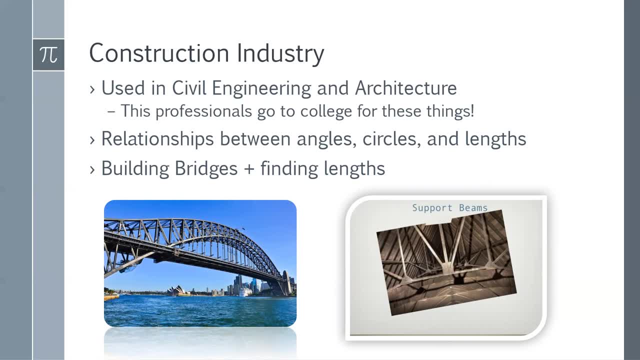 load, maybe roof slopes, and also the placement of lengths that are used for supporting beams. So, as you can see- on the right there's a photo that shows that- And another thing that they also do is finding out the angle the sun hits the structure. So in this case, this: 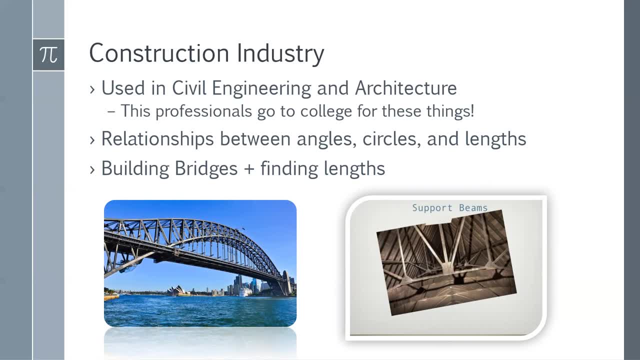 can be applied to the bridge. that's shown. So, as you can see, there's some sort of sunlight coming on and the architects and civil engineers had made sure that there is a good amount of sunlight and not too much hitting the bridge. And, additionally, we can also see that trigonometry was used to create circular shapes as well. 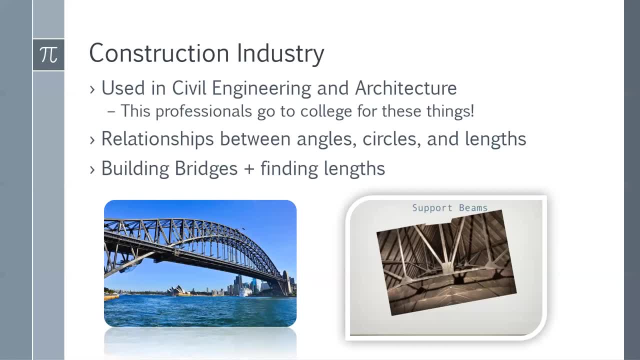 So, for example, in this bridge again, we can see the circle shape or an oval or a semicircle, and that was really good as well. And to also find the length and basis we need to use trigonometric functions such as. 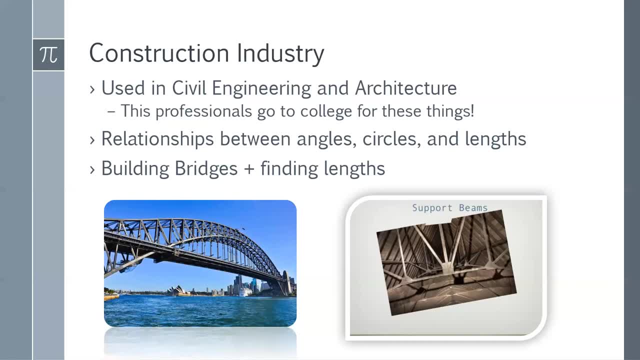 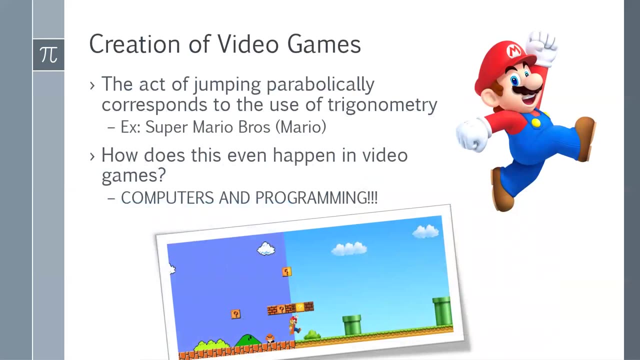 sine and cosine to find the height and distance of a building, And this uses the idea and concept of a right triangle. So therefore, we could see the importance of trigonometry in the construction industry today. Now we'll be talking about the creation of video games, So I know a lot of you guys play 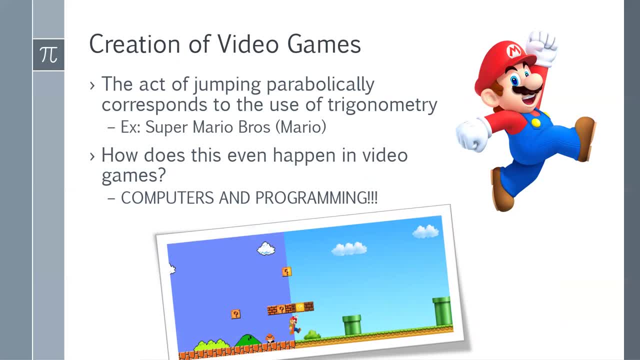 video games, And the use of trigonometry is really important in games. So I'm going to show you how to use trigonometry in a video game design, because without this, you'll only be able to jump vertically. Now, thanks to Hipparicus, we have the ability. 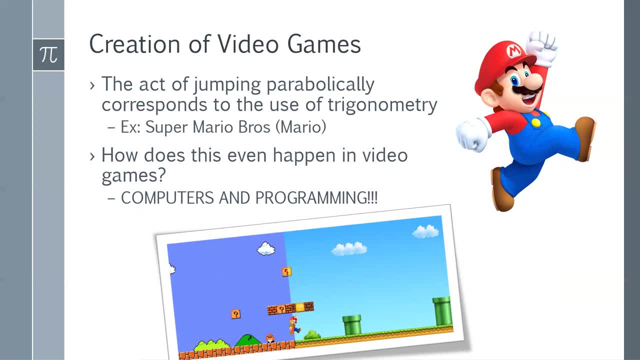 to make characters jump parabolically. One great example for this is the game Super Mario Bros. So in Mario you could see him effortlessly gliding over these different roadblocks, and he doesn't quite jump along the y-axis. He takes this slightly curved pathway to avoid the obstacles that are in his path. And Mario 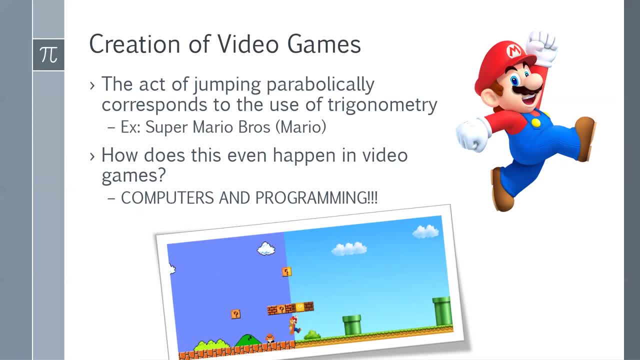 is able to do that thanks to trigonometry. In fact, the only reason that this occurs is because they're created by IT and computer science professionals. Now, when they are coding these games in the front end and back end, they have to be mindful that the character is not jumping up and down or along the y-axis. 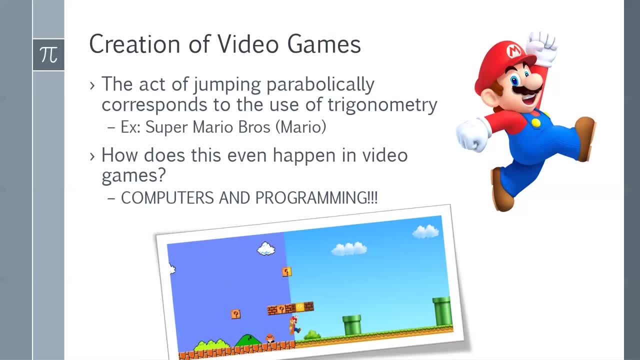 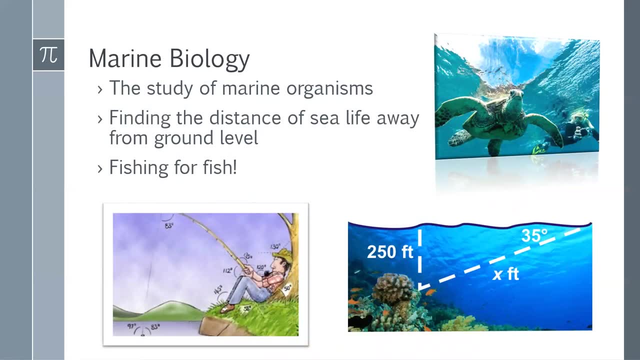